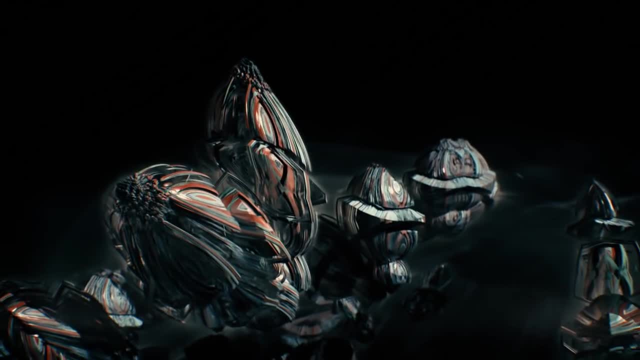 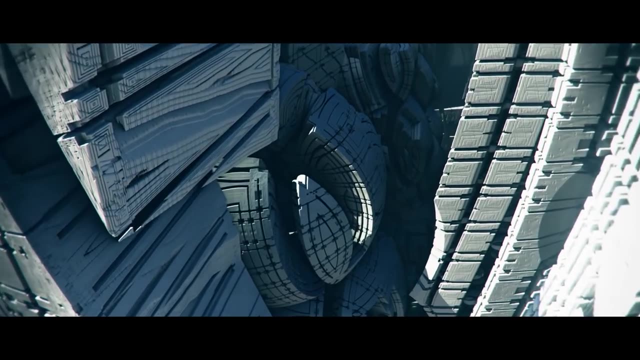 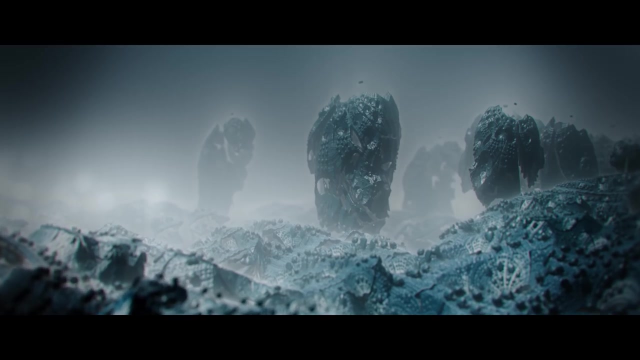 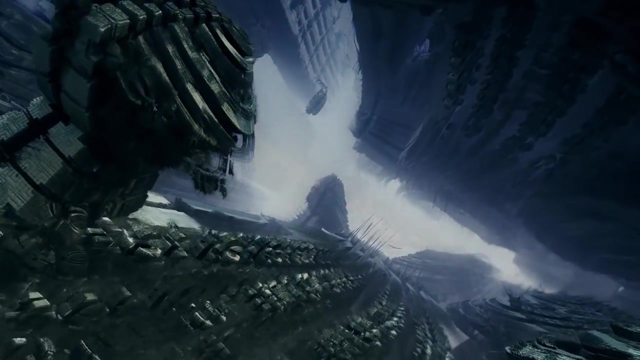 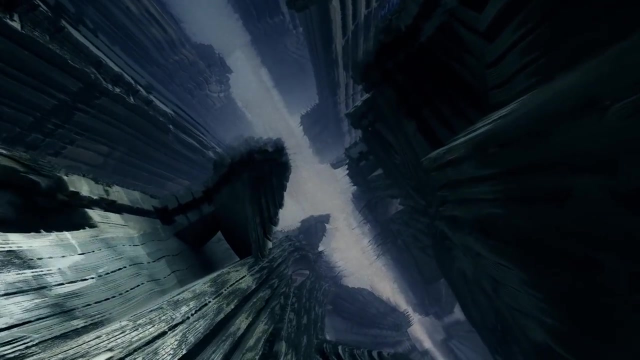 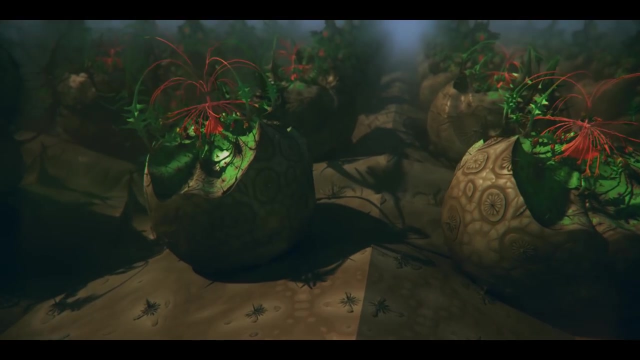 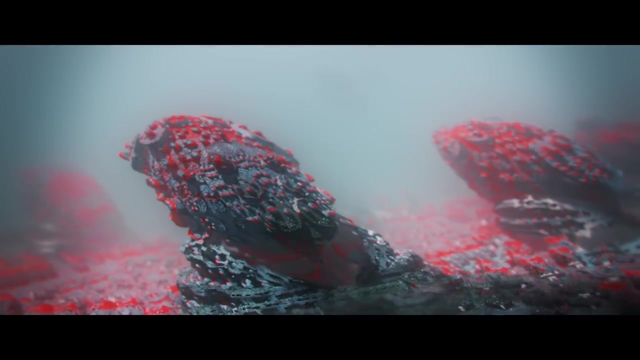 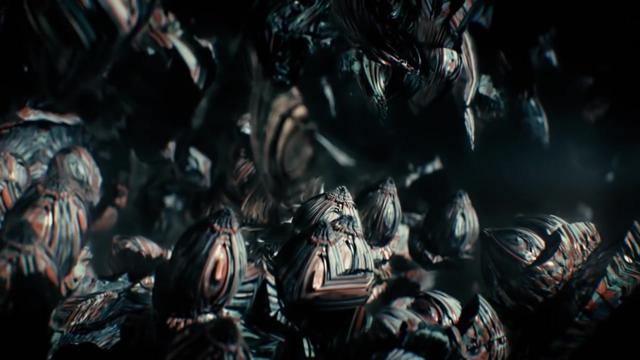 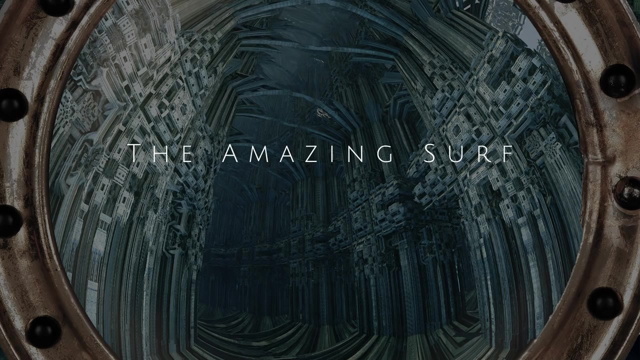 They're defined by the fact that they have a cluster of matter and there's usually some space in between. So they're really clusters of parts And they come in lots of shapes, but I just call them parts. These are called the. So the Amazing Surf. 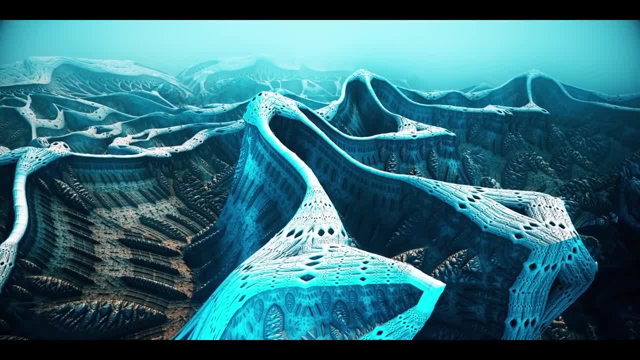 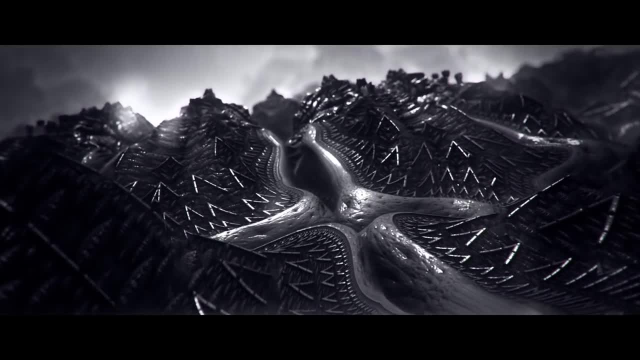 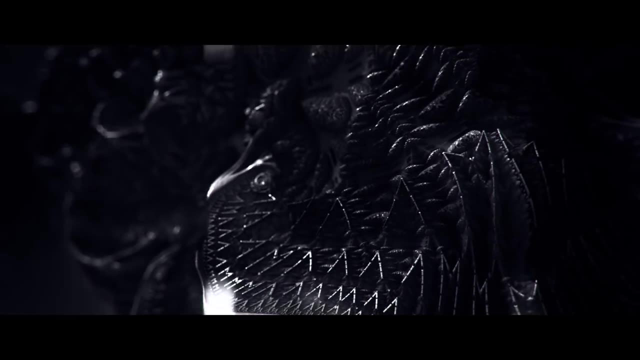 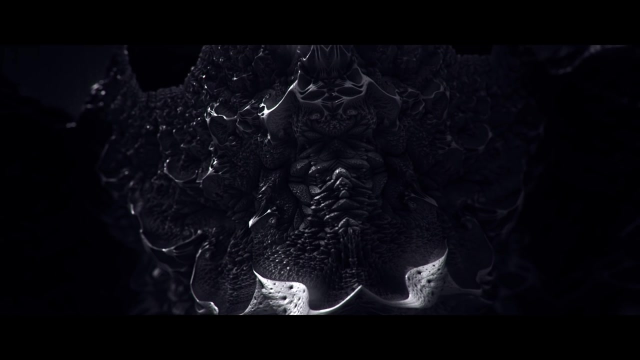 is a amazing circle of objects, a amazing surface. I guess that's what surf stands for. it's a surface, it branches and although it can manifest itself in many ways, sometimes you get to see the tree like branching structure. sometimes only the edges are visible, but most of the structure seems to be made up by the ends of an infinite branching. 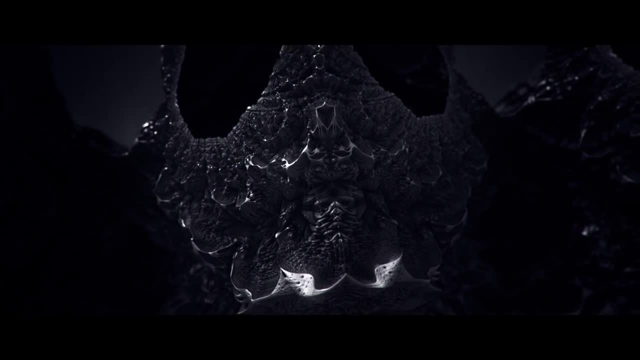 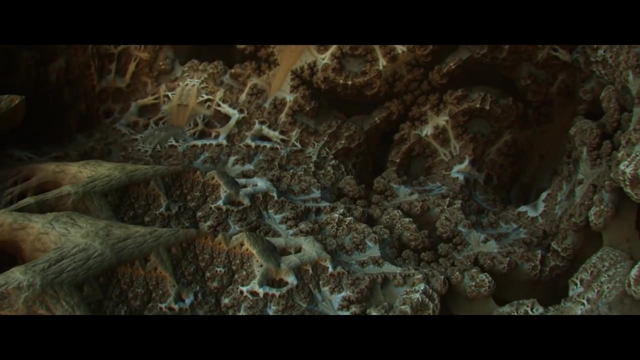 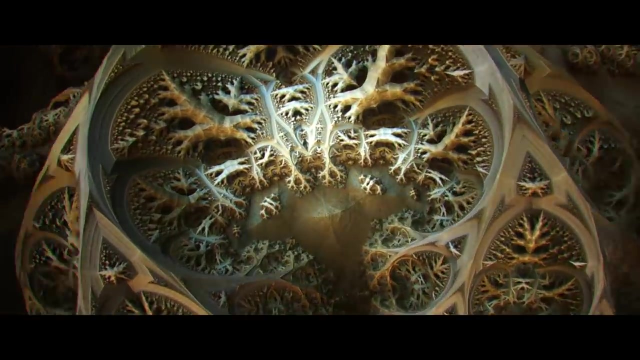 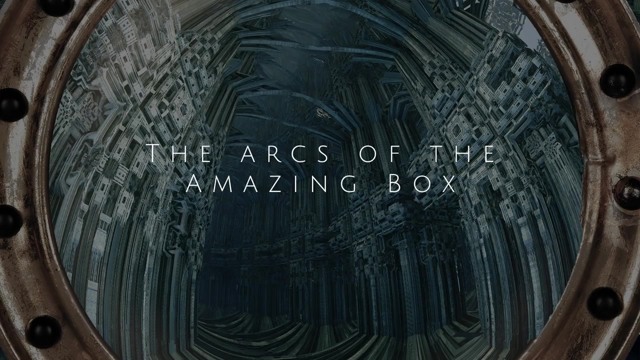 tree. so whenever you see this branching pattern, you see like a big, like a stem, and it branches into two and four and sixteen, thirty two and so on, and then and the very infinite, and it creates this surface. so the amazing box also comes in many different shapes, many different forms. 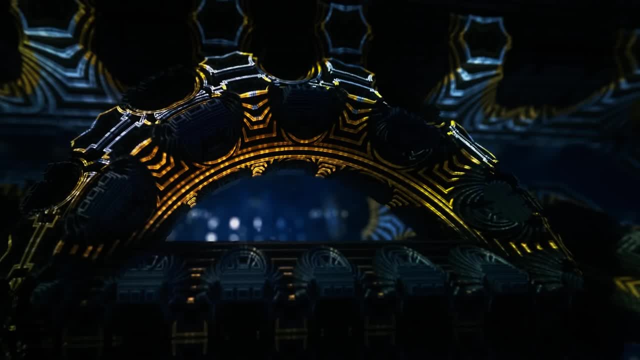 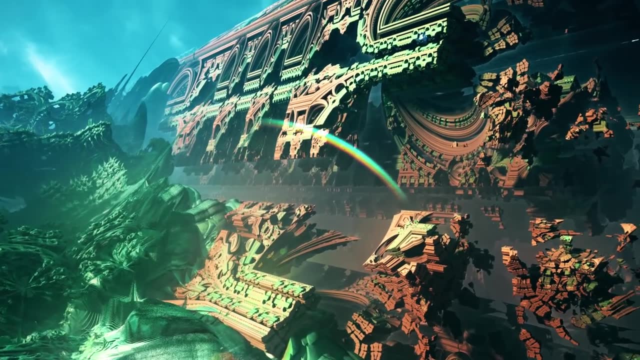 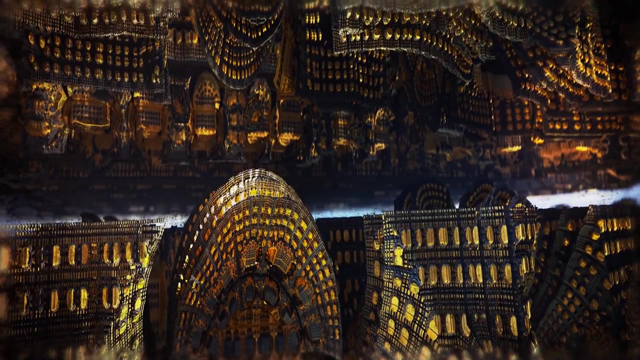 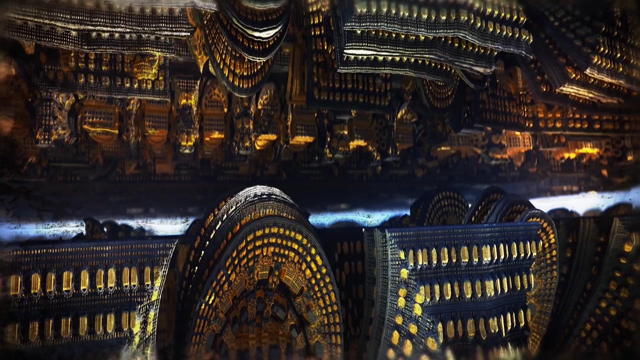 and it can be combined with other things, but it's always characteristic. you can always see its arcs. they really stand out. you can recognize them by one side being arc shaped and the other is flat, and I've seen the structure many times, many different forms, and sometimes they can really be beautiful and sometimes not. they kind of sometimes look like. 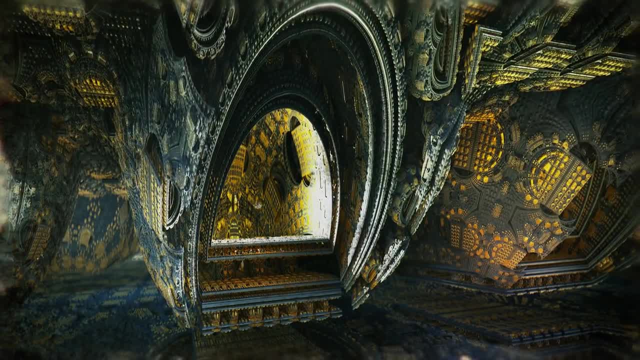 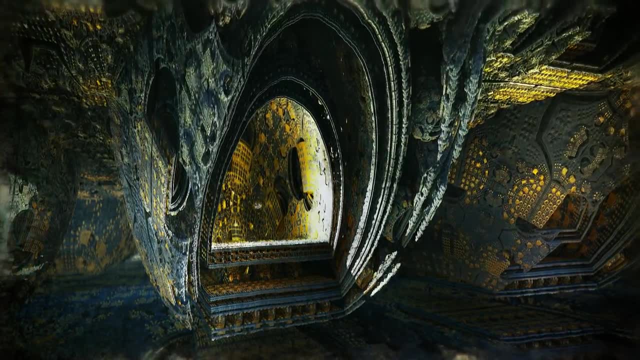 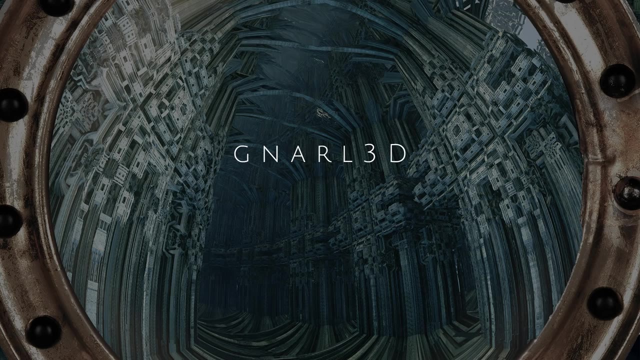 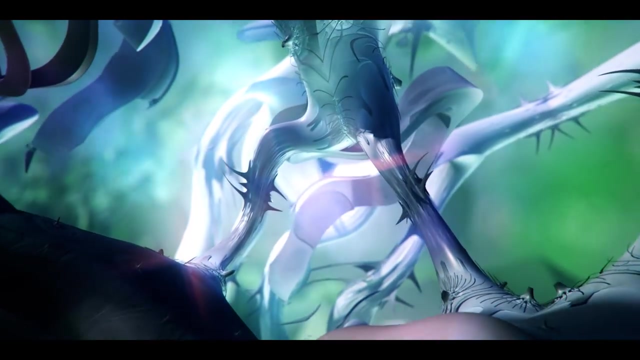 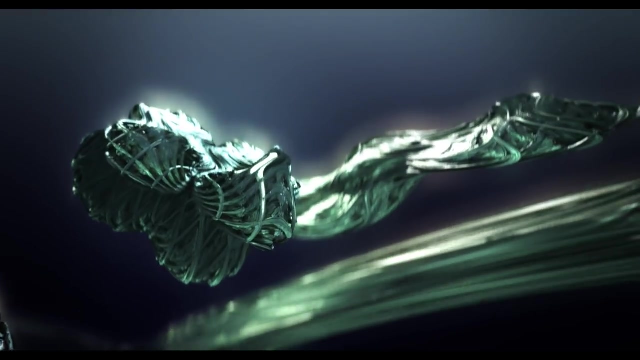 like big windows from a church or something like that. it's really quite pleasing to the eye. so Gnarl is probably one of the most easy concepts to grasp. Gnarl just deforms the world into a wavy world. you can see it. the waves operate on different levels and matter can. 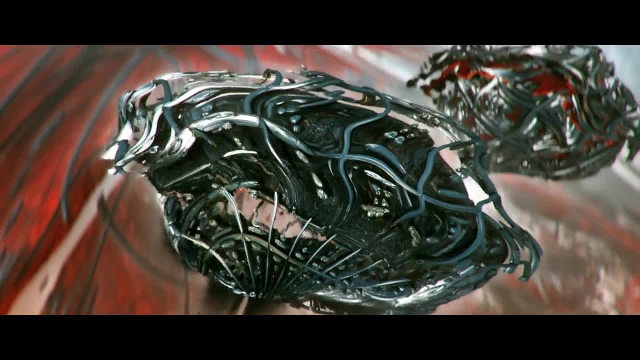 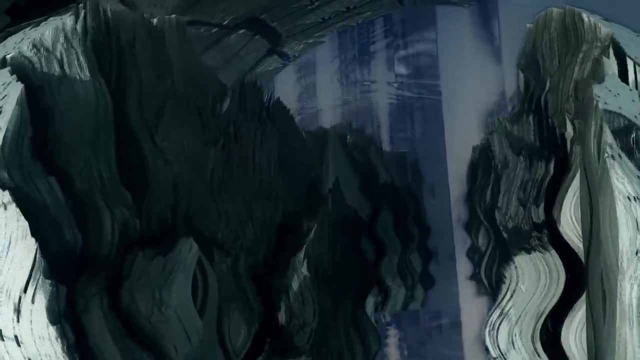 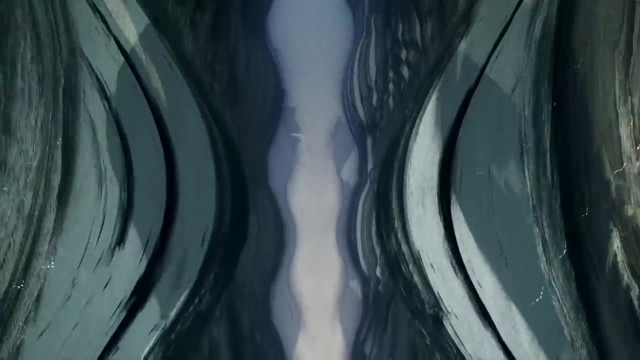 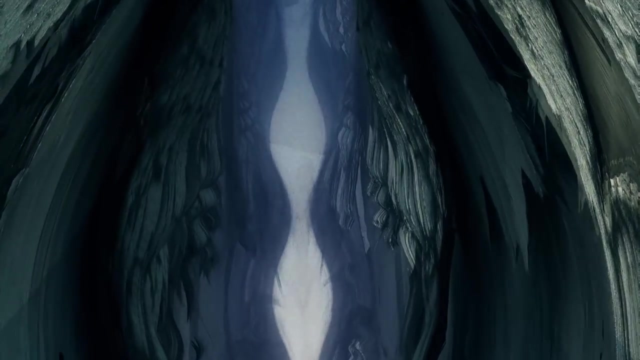 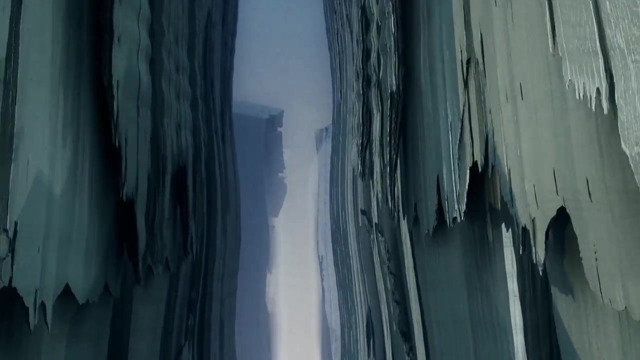 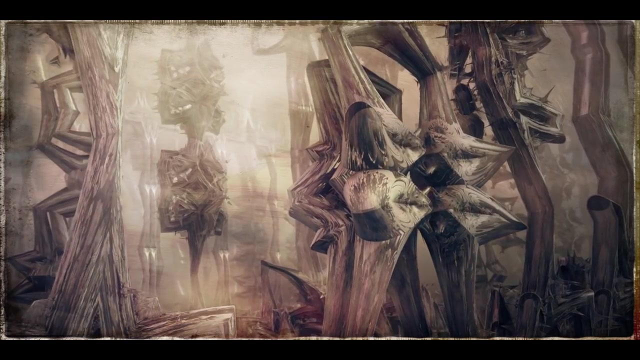 swim through the predefined wave as well, so they're slow to render, but they can look really awesome. so, like a straight line becomes organically wavy and it can have some really interesting effects. Min R or Minus R as I call it. I'm not sure if min stands for minus. this is a crazy parameter. 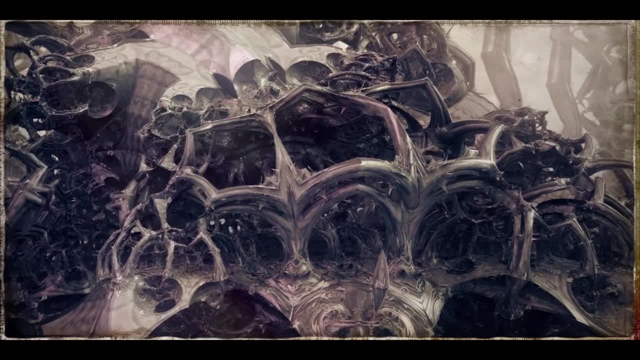 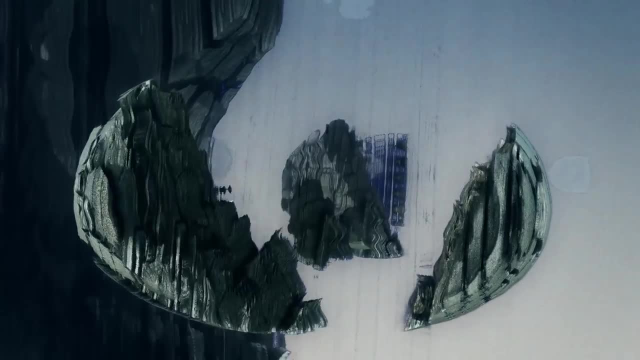 you can find in many formulas such as amazing boxes and surfaces. so sometimes it completely remains a mystery. so the minus are: will have stuff just like matter, just disappear into into sheer nothingness, alright, and sometimes you can like see and you can kind of go: what are you doing here? you're running out of thing to play with it. you just keep playing with it, like trying to figure out how you're going to do that. so, and you know, if you're going to stop playing this, then we'll play this music and then we're going to have a little dance with it. I don't know why I'm doing this. 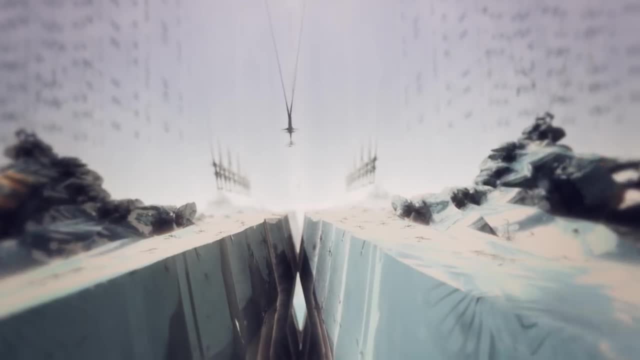 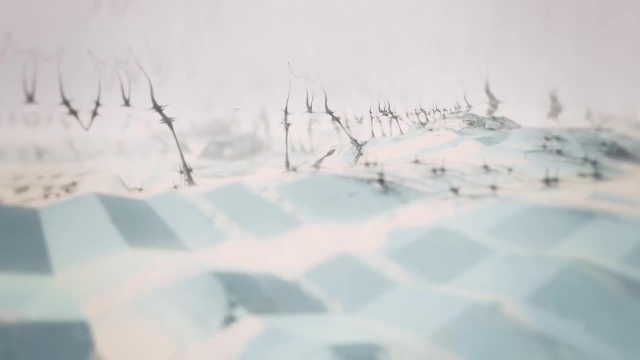 this book, that which is going to be sort of a new, sort of a kids song or a new music. so it's that it is just like a little bit of an extra performance and- and I think that going to, Sometimes you can see the sphere, the three-dimensional sphere, around the empty void that is sucking up the minus-r stuff. 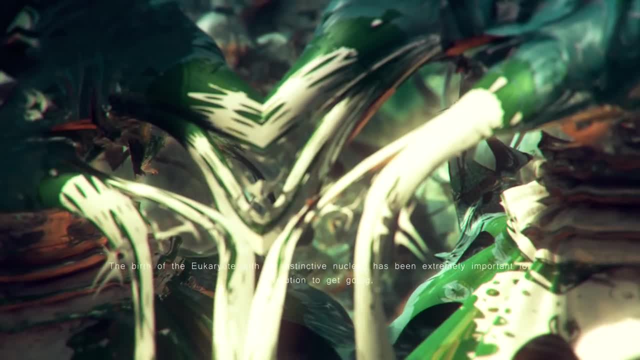 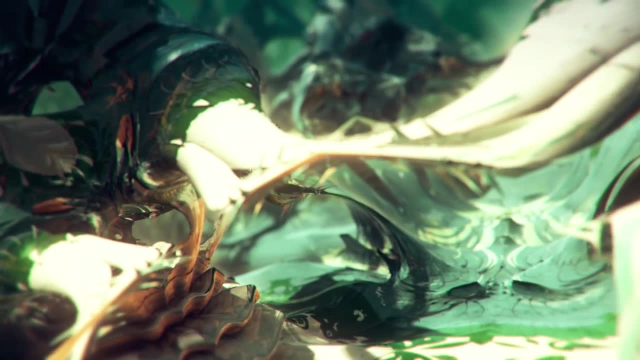 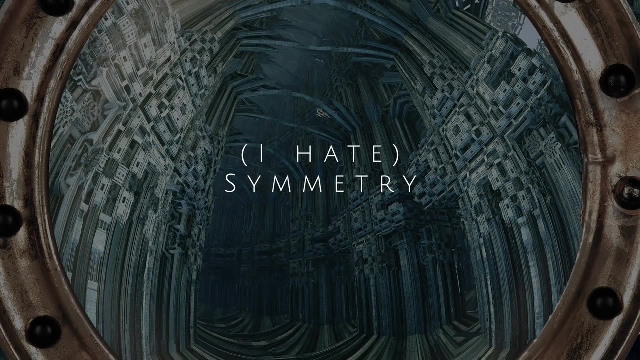 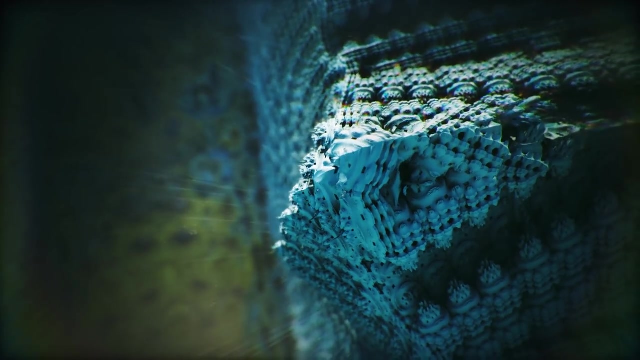 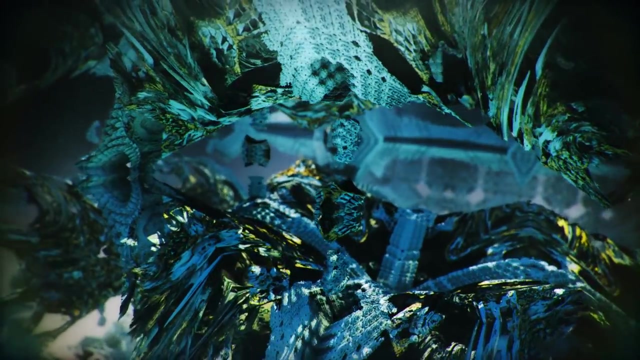 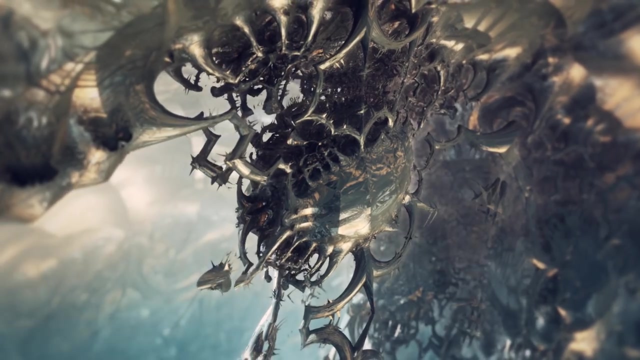 Maybe like the Terminator robots when they travel through time. Uh, symmetry. So I hate symmetry. I don't like. it's maybe weird, but I don't like the fact that things are symmetrical and I try to avoid it, But it's a fact of life in the fractal worlds. So they seem to exist everywhere, symmetry axes. 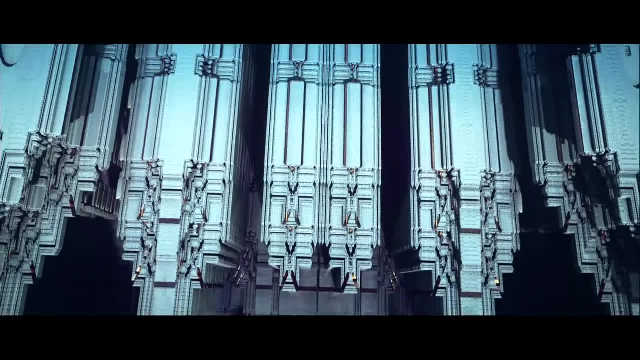 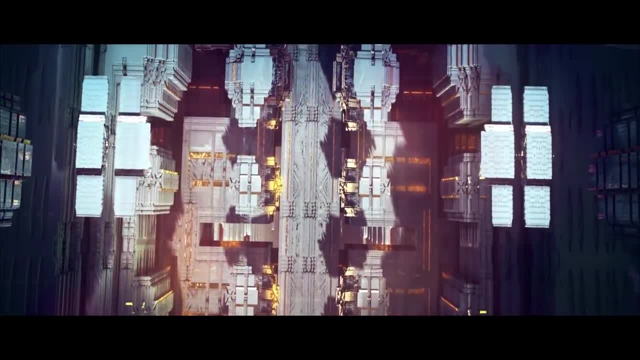 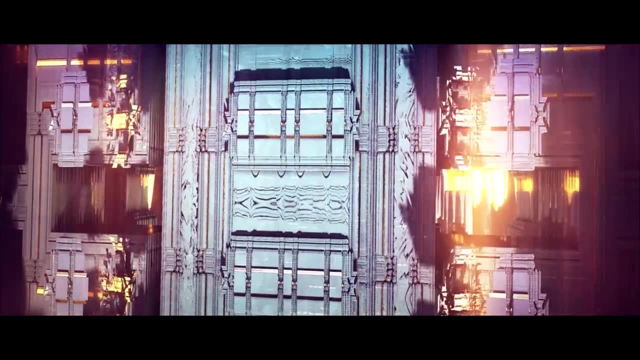 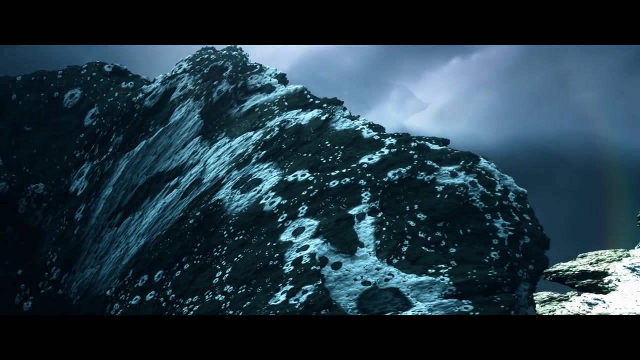 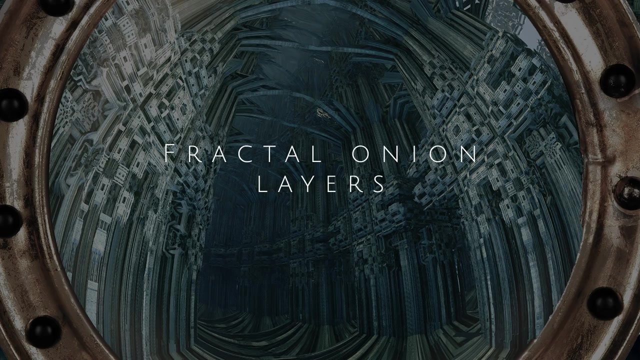 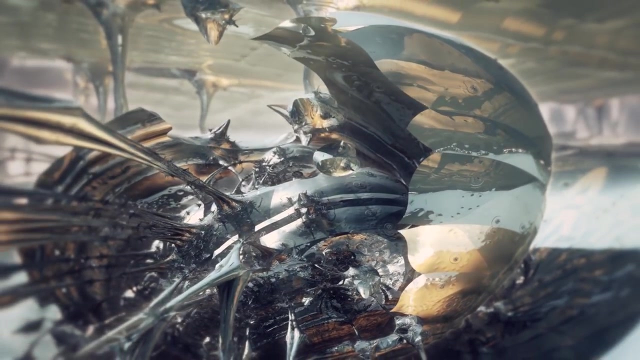 And sometimes they make matter disappear or reappear like quantum particles that cancel each other out. I don't like it when it happens, but it's just a fact of life, And these are some examples. Some fractals are more like solids, but others are like onions. 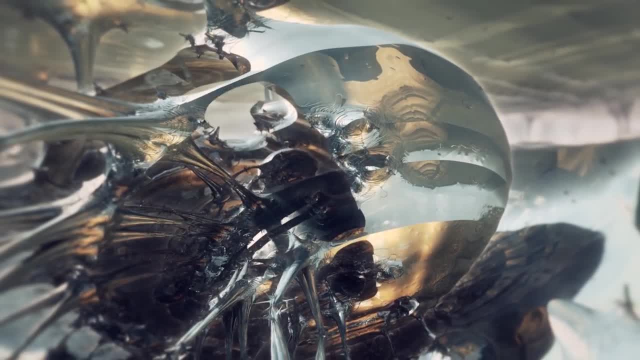 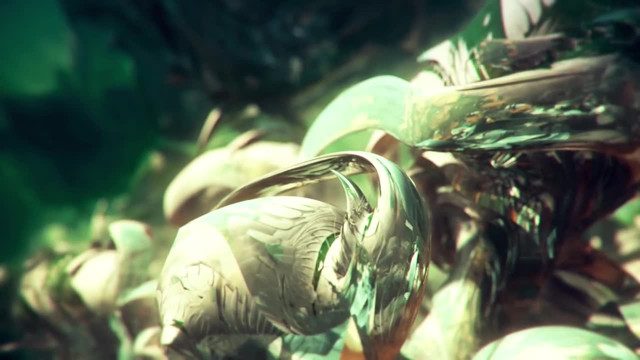 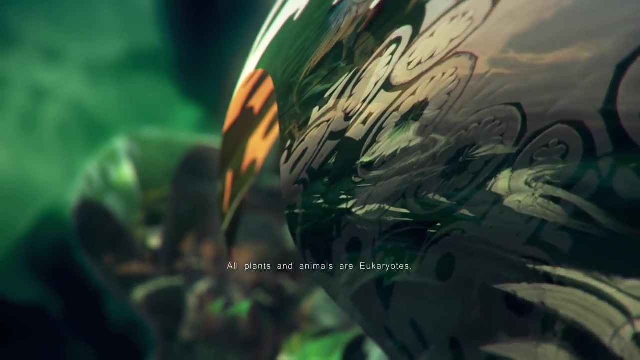 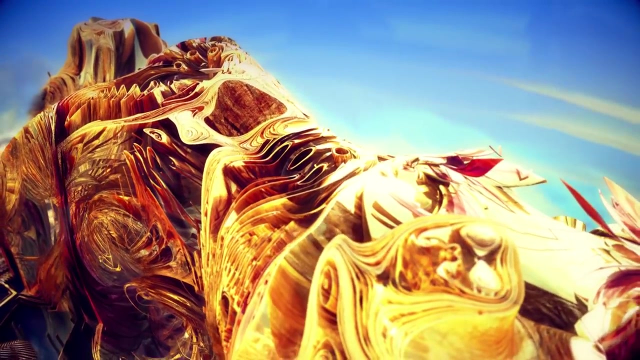 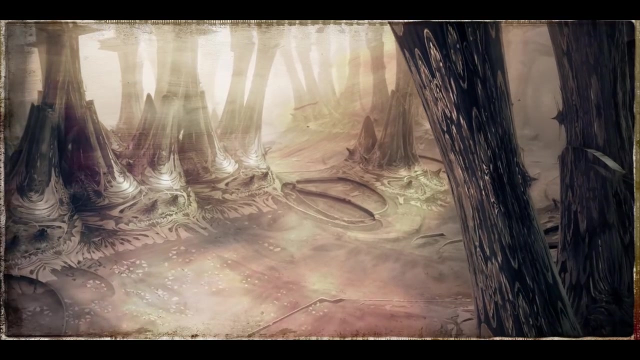 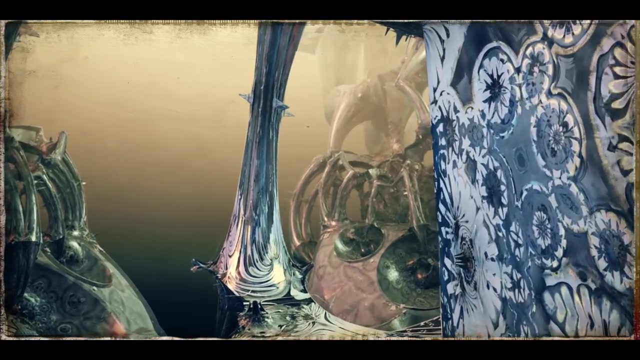 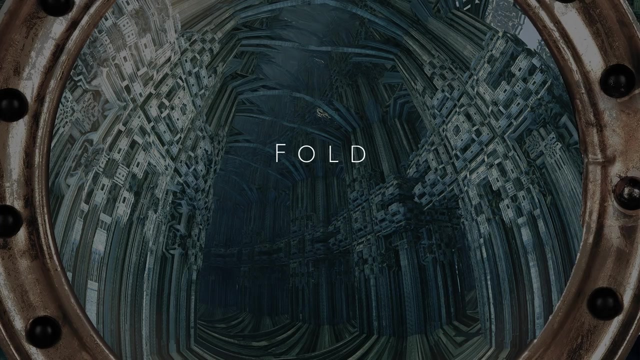 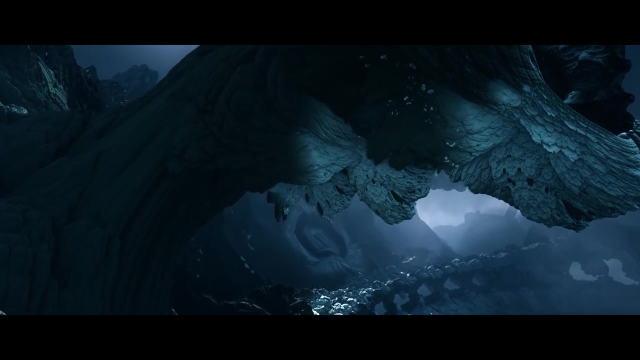 They're like onions. They're like onions in a way that they have lots of different layers And you can sometimes grow another layer on top and you'll get a different shape, like a different pot. So the fold parameter is by far one of the most interesting ones. 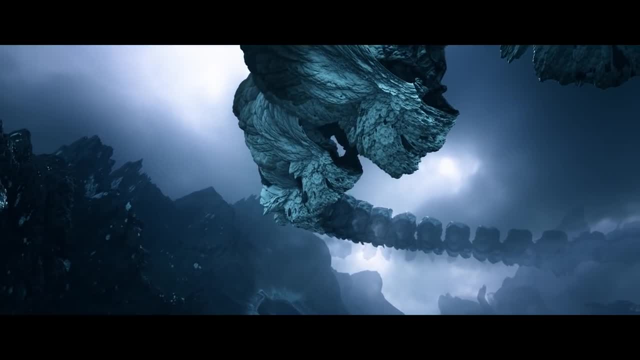 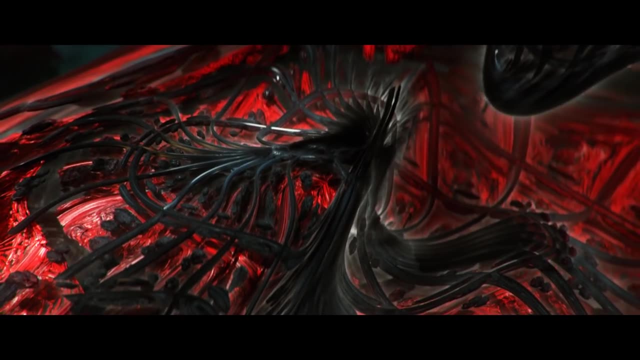 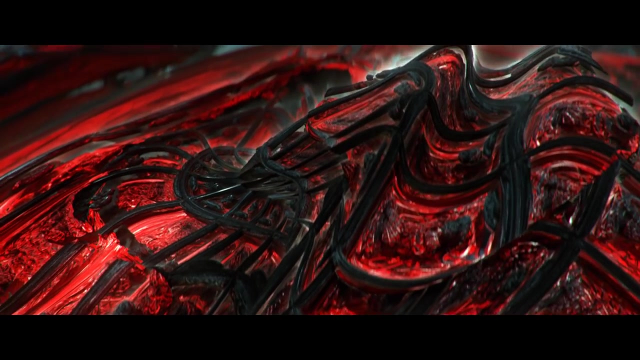 And it will have many different kinds of effects, And I hope that this will give you an idea. Matter sometimes comes together and it seems to fuse or it seems to move apart, Not like the minus R one where it just disappears. Here it's more like it separates and it flows through space. 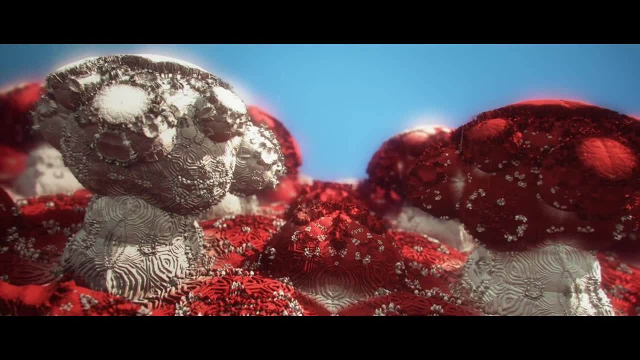 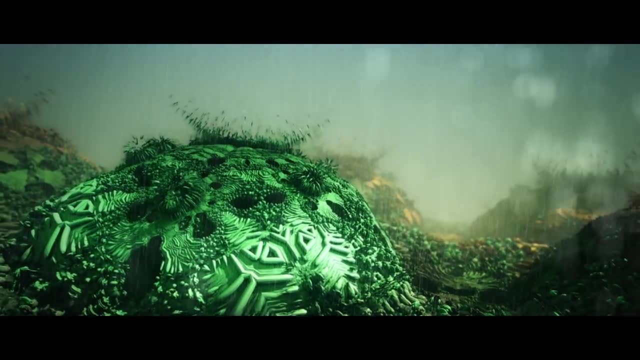